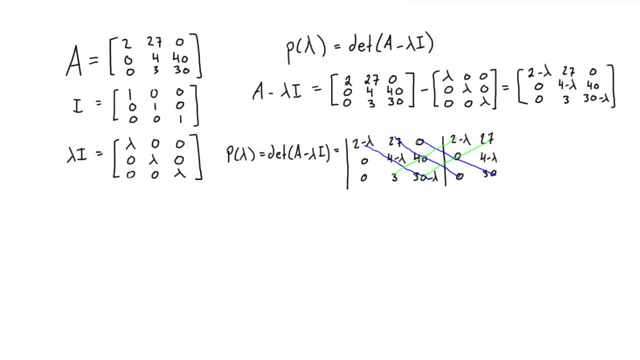 other way, from top right down to bottom left, and we subtract the products of each of these and that's just going to be a bit of a faster way for us to find the determinant of this matrix. that is a minus lambda i. so if we write that out first of all for the blue lines, we get this: 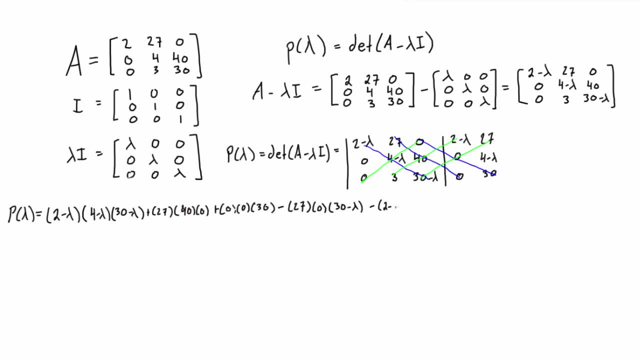 and then when we go through and do the green lines, we get the next three terms, and when you have matrices that have zeros in them, then typically a lot of these things are going to cancel out. so we have a zero in this term, it goes to zero. that looks like a six. 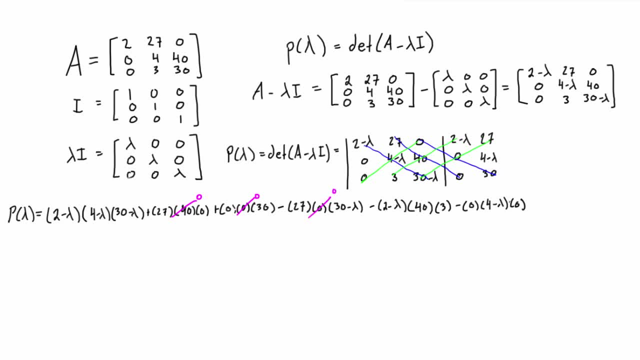 it goes. this one goes to zero, this one has got a zero and this one also goes to zero, which makes our life a lot easier. so if we take this one step further and simplify the remaining terms, which is just one term here and one term here, we get this, and then we can distribute this last set of 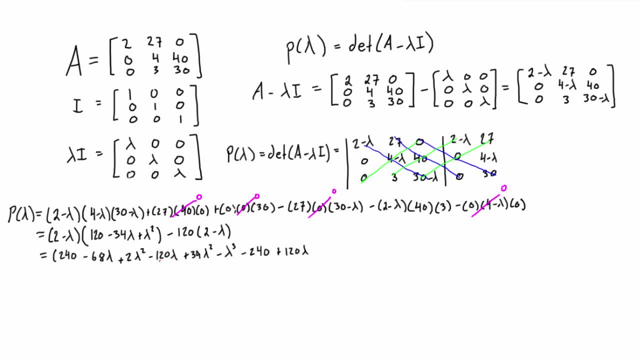 brackets and again, a lot of stuff here cancels out. we have negative 120 lambda and positive 120 lambda and then negative 240 and positive 240, and i guess i opened the bracket there so i probably should have closed it here. but either way, it actually doesn't really matter. we can actually just get. 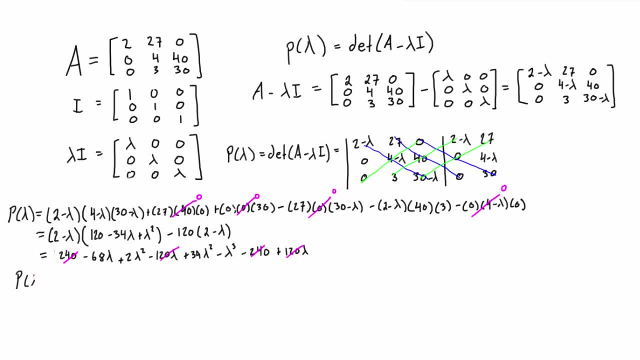 rid of those brackets for now. so when we do the final simplification here, we get negative lambda cubed plus 36 lambda, squared minus 68 lambda, and this is the characteristic polynomial of a. so if you're looking for a specific Michigan signal that the general professor is looking for, then you. 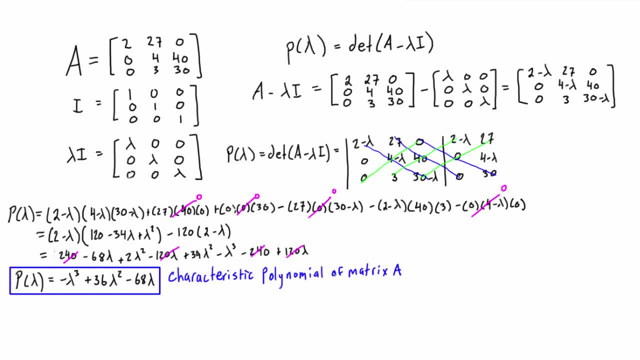 can put a box around it and stop here. but often the reason we're even finding the characteristic polynomial of a is because we're after the eigenvalues and eigenvectors of a matrix. so basically, if we just set the characteristic polynomial of a equal to zero, then we call it the. 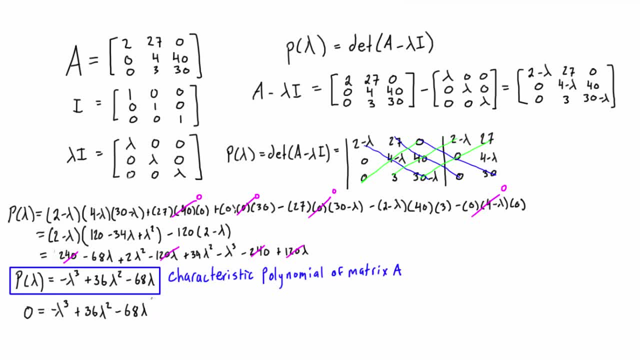 characteristic equation and if we can find the roots of this equation, then those will be the eigenvalues of the matrix. so if we just simplify it in a few steps, we're going to find that the roots are 2 and then in this, frequencies of the nature wird. 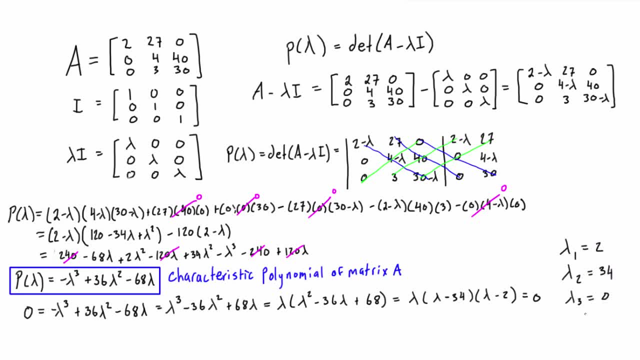 34, and 0.. And these are the eigenvalues of the matrix, And so if you were also looking for the eigenvectors, then we could use these eigenvalues to calculate those. But this video was just really about finding the characteristic. 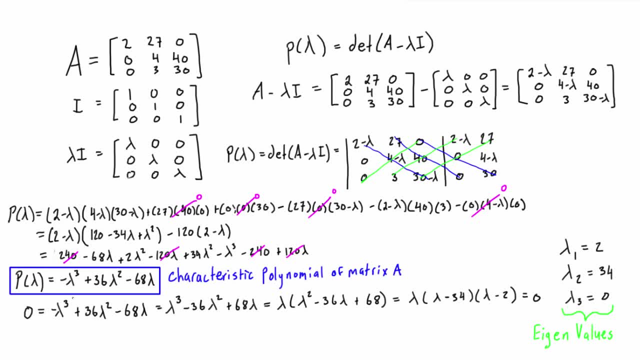 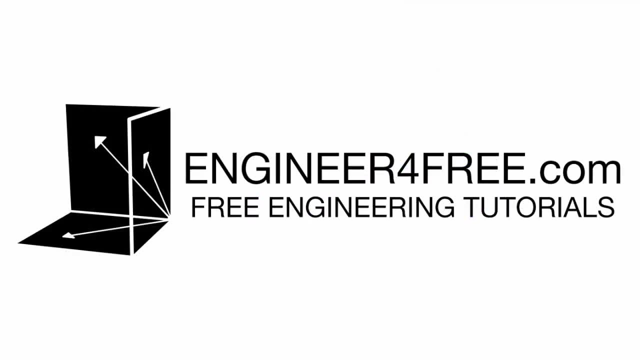 polynomial of matrix A. And so if you get to this step here, where we have the blue box around it, then you will have found the answer to the problem of just finding the characteristic polynomial of the given matrix.